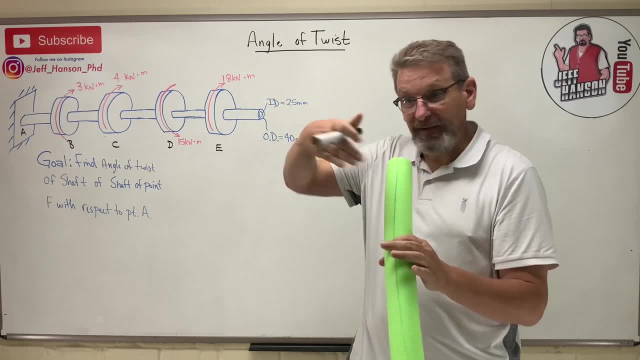 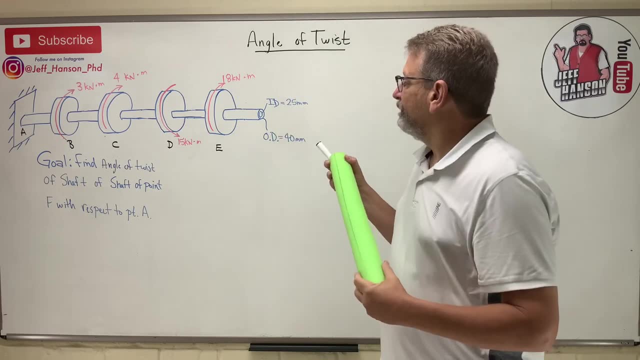 and then the other end, I twist it back the other way. that angle of twist may go down the shaft, not in a straight line there. right, I would twist it the other way, but I only have two hands, So I've got a little problem here for you. that's going to demonstrate. 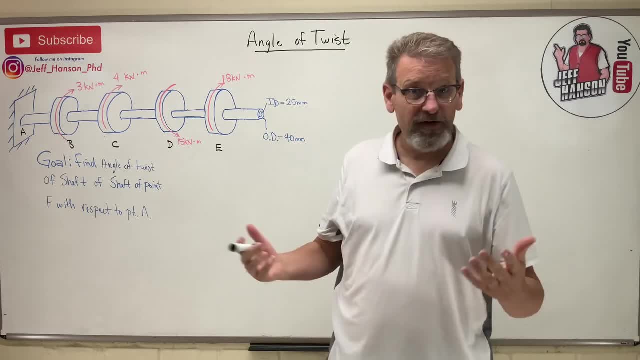 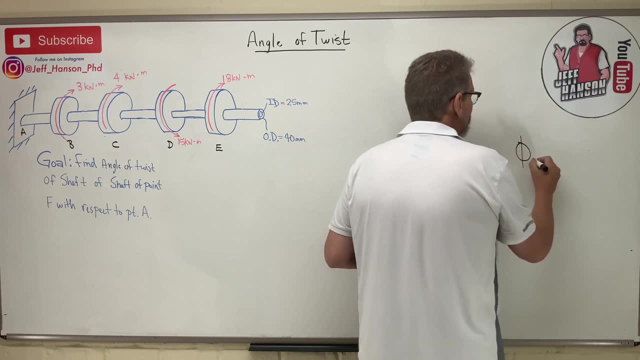 that, And so the way I want to do that. well, we got a new equation, don't we? There's a new equation for the angle of twist, and the equation looks like this: V is equal to TL over JG. okay, 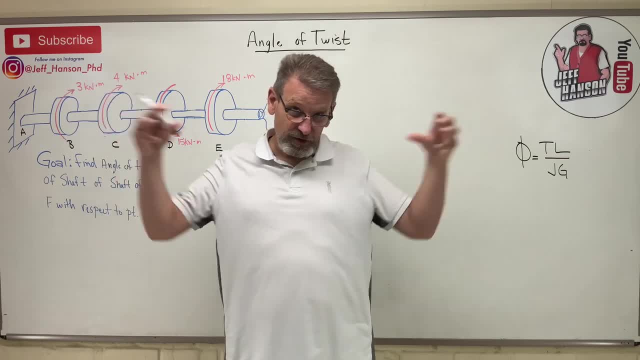 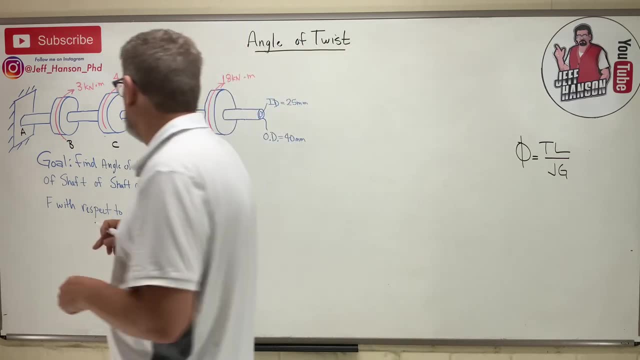 Now, the longer that shaft is, the easier it is to twist. If it's really short, it's really hard to twist. So let's look at this shaft over here, Let's make up some numbers here, Let's say that. 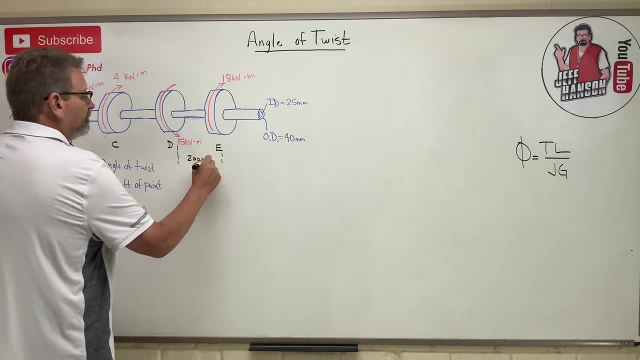 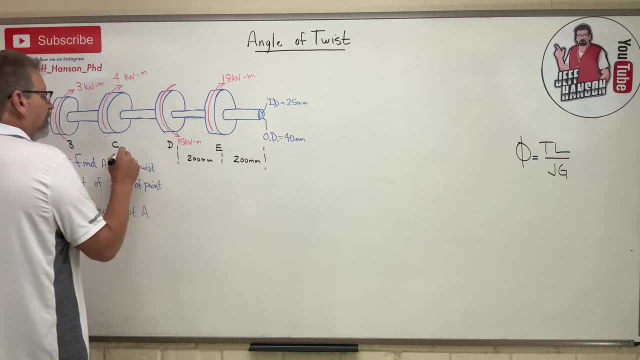 this is 200 millimeters. This can be. that looks like 200 millimeters. This looks like 300 millimeters. We're just making this up. This one's that's even farther, that's 400 millimeters, and then back to 200 over here. 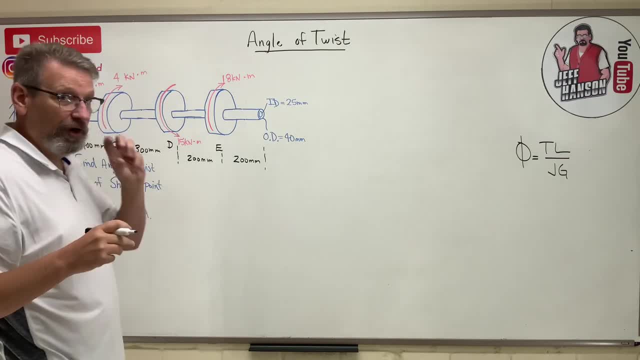 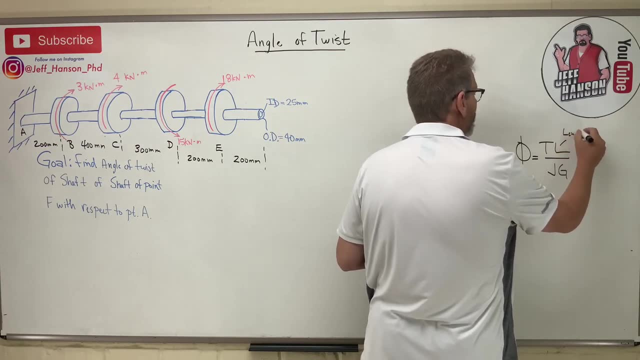 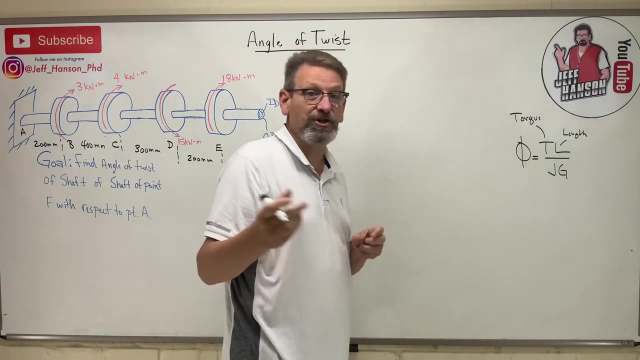 Okay, So the length of each shaft really matters on that angle of twist. So this is the length of the piece in question. Okay, This, of course, is torque. And we know how to find the torque in each section, don't we? 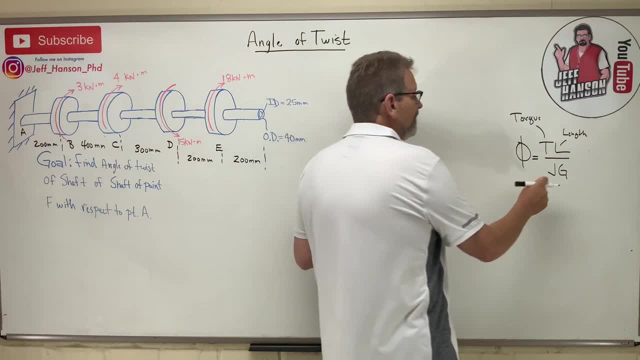 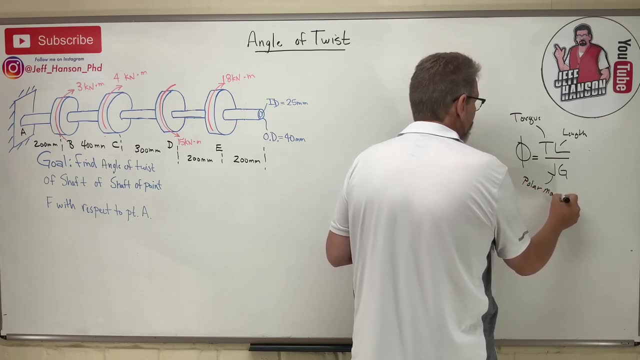 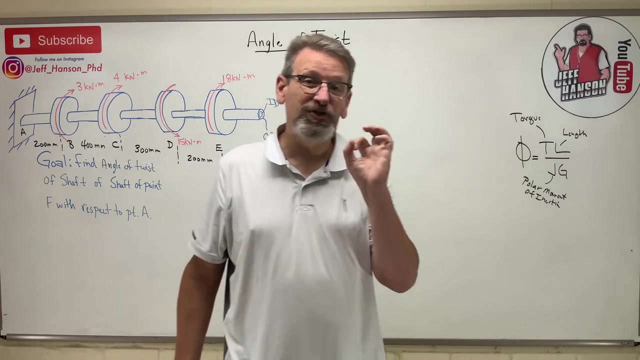 We'll do that here in just a second. And then we've got J, which we know J also. That's the polar moment Of inertia. And remember, the polar moment of inertia is different for solid shafts than it is for hollow. 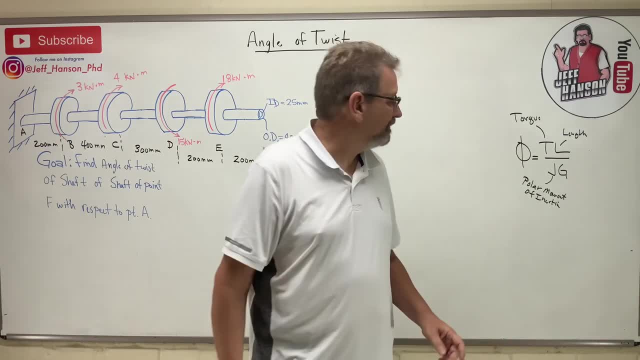 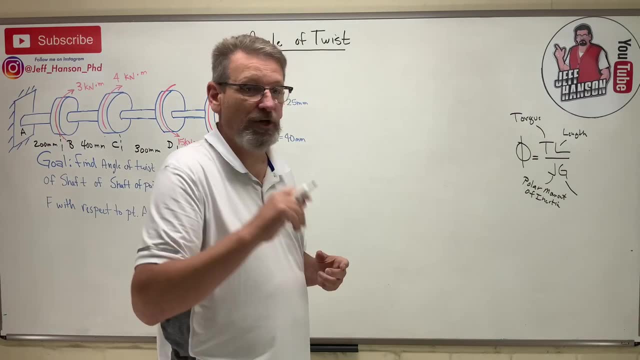 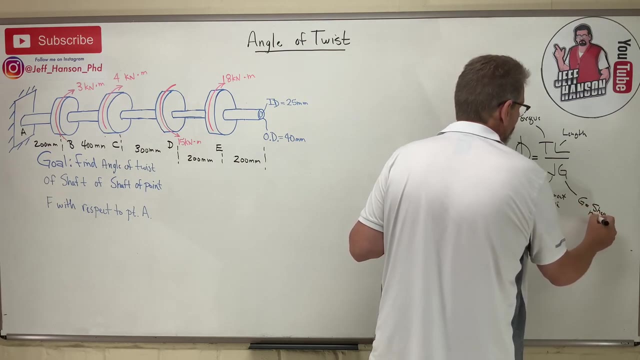 shafts, And here we have a hollow shaft. Okay, And then G? what is G? Well, G, we know. G, That goes way back, doesn't it? That's the shear modulus of elasticity, Okay, Of elasticity. 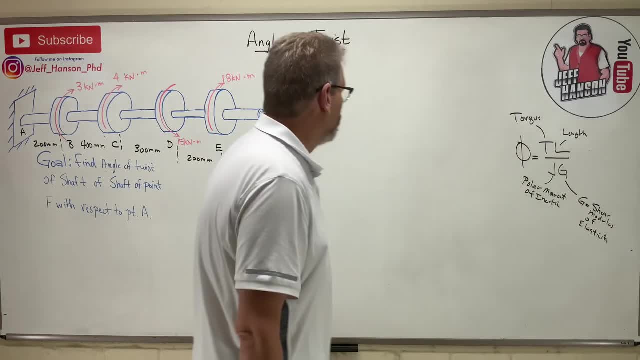 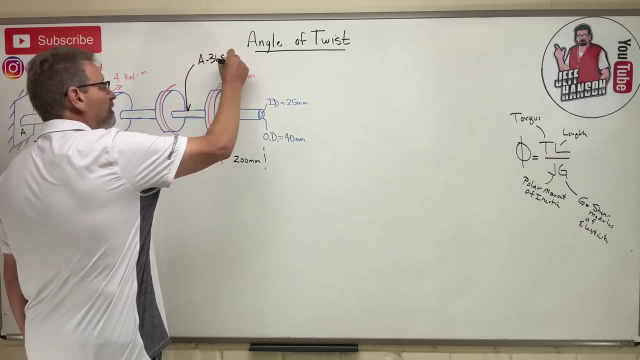 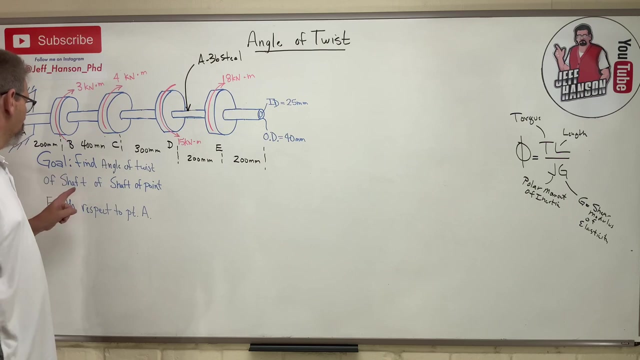 Of elasticity, G for angular force, And that is a look-em-up. So let's say that this is made out of A36 steel. Okay, Can we find the angle? that wants to find the angle of twist of this shaft. Well, I got too many shafts in there. Shaft of point F with respect to point A. So here's point. 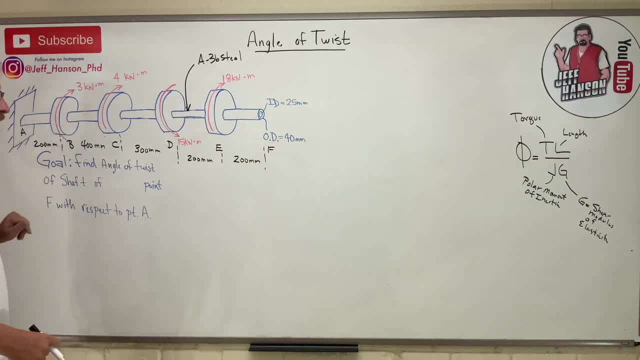 F way down here on the end. And here's point A, And here's point A, And here's point B, And here's point A is kommt in here Herrnkel, French Commentator a, at the wall right. so all these different torques applied and imagine this thing over here has a. 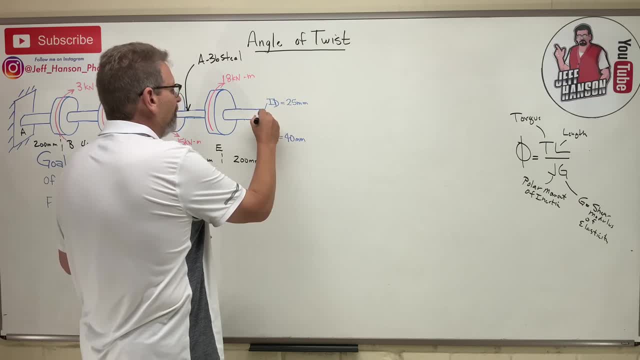 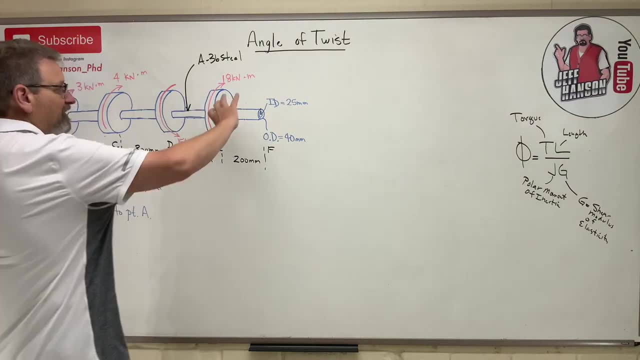 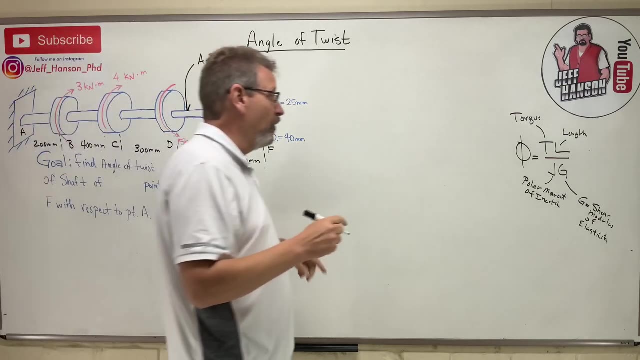 imagine this as having a a little clock dial on it, right, and it's straight up initially right: it's at 12 o'clock. so, as i apply all these twists, does that, does that move um clockwise or does it move anti-clockwise from there, and how much? now one thing you need to know about fee. this is important. 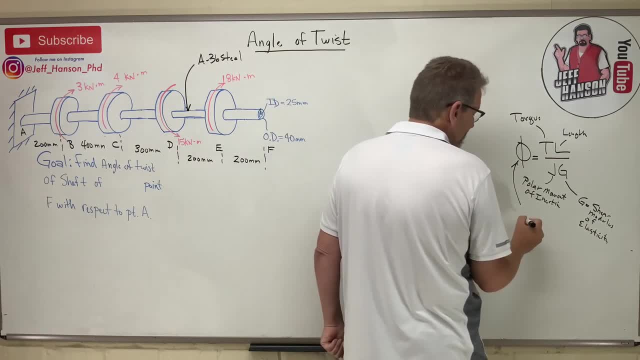 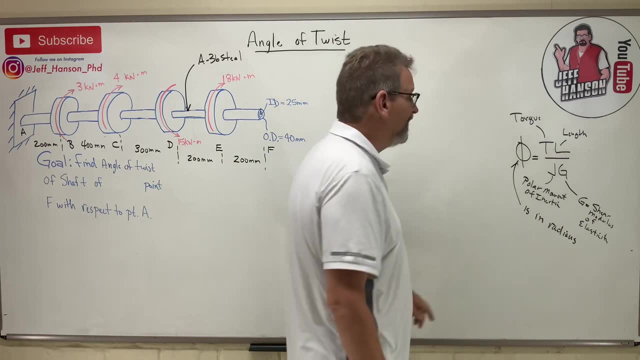 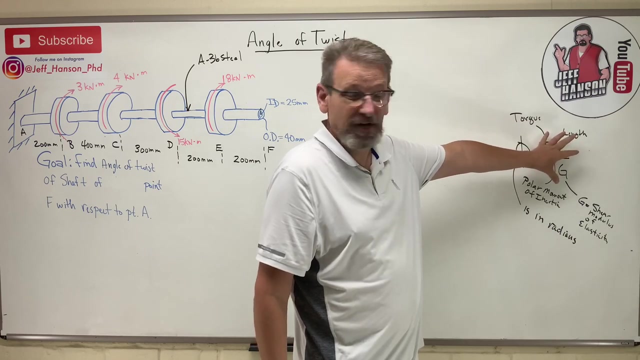 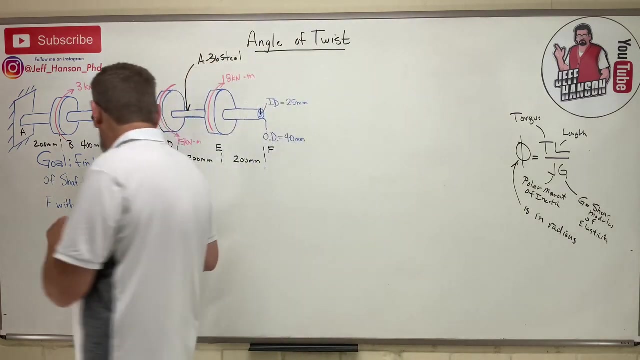 muy importante is that phi is in radians, okay, which tells me that once i put all these units in, for all of these variables over here, everything should cancel out. radians is a unitless number, right? so if you want it in degrees- and let's do that- let's make it in degrees. let's say in degrees. 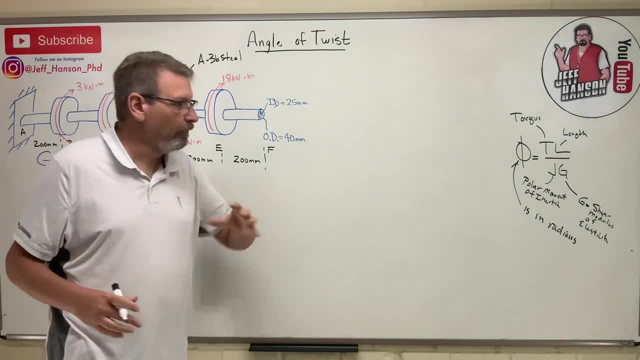 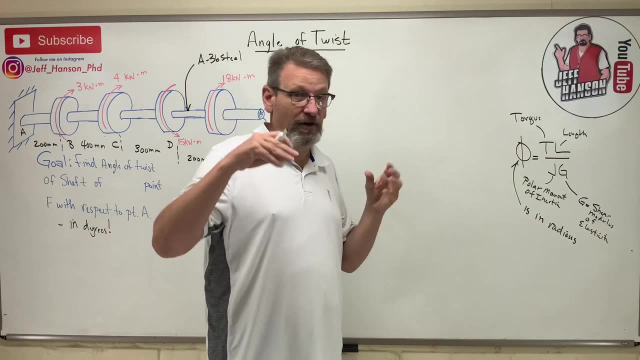 okay, let's just do that, so we can just practice one more thing: at the end we'll have to convert it from our answer in radians to degrees, and then we'll say: clockwise or counterclockwise. now, everything that we're going to do is going to be referenced from. here's your eyeball looking at the 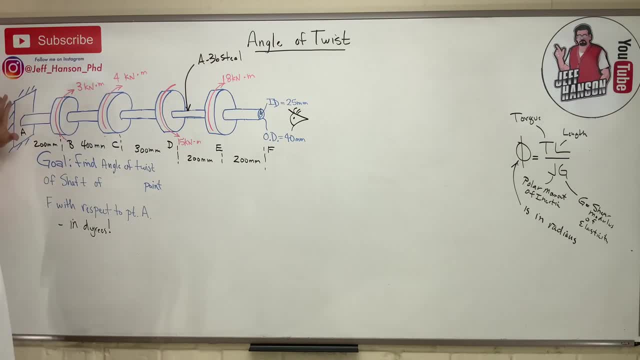 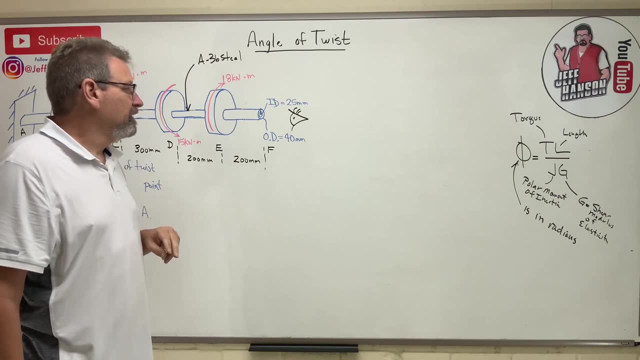 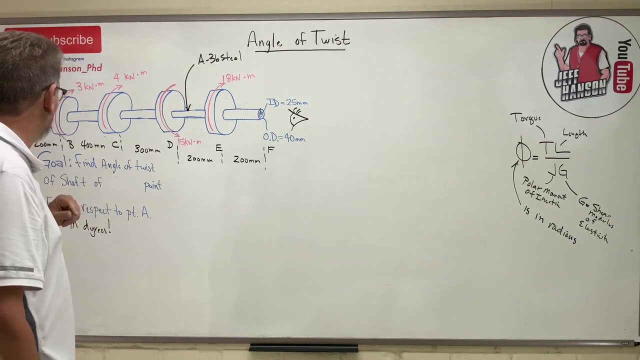 end of that shaft. okay, so point a welded to the wall, point a, our point f is just out in space. it's free. okay, so let's call. i don't know. let's do it like normal, right? let's? uh. let's do counterclockwise as uh. 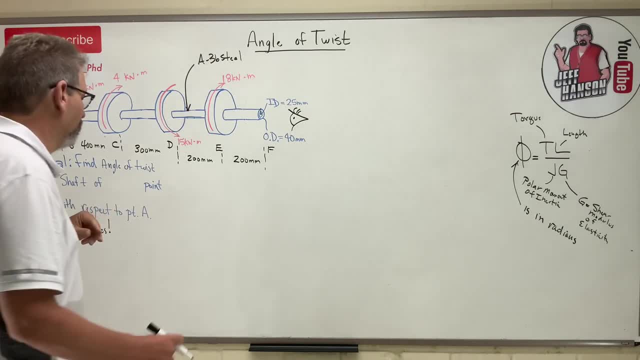 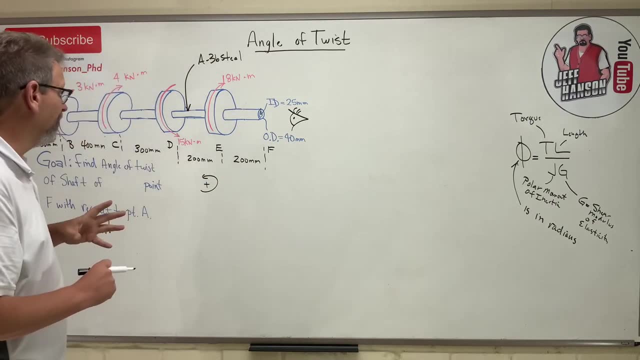 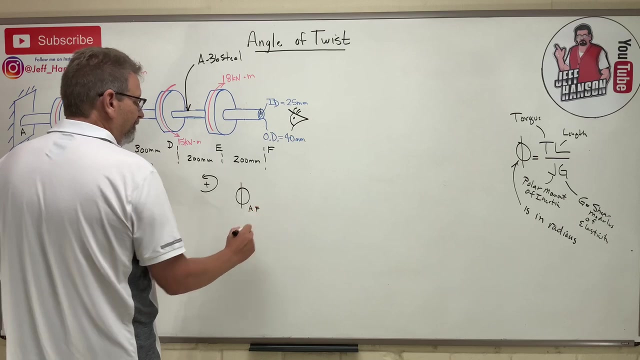 as positive and clockwise is negative. that's what we're used to, right, okay? so counterclockwise is going to be positive, okay, and what we're going to do is we're going to add up. we're going to do this. phi for a with respect to f right is equal to the angle of twist in section. 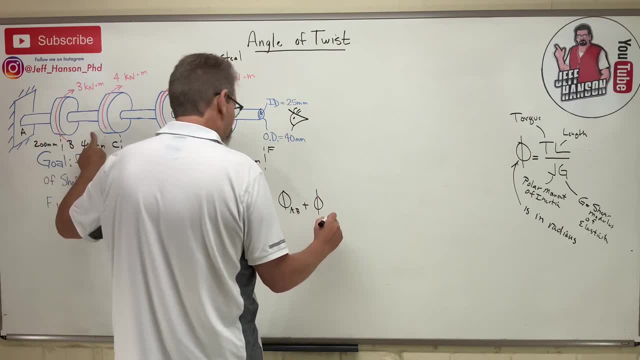 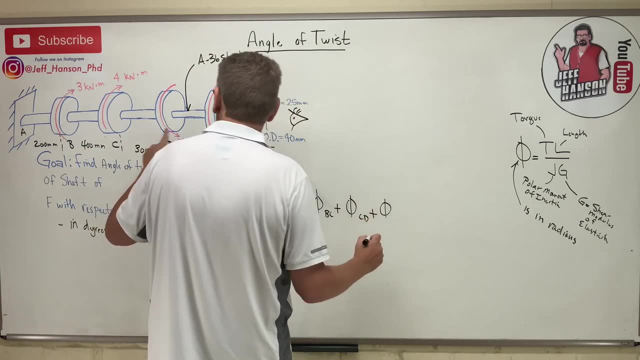 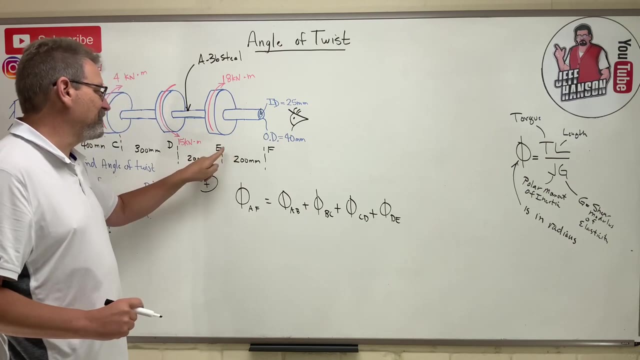 a, b plus the angle of twist in section b, c, plus the angle of twist in section c, d plus the angle of twist in section d, e, and then is there going to be any angle of twist in section e- f? is there any torque in section e f? right, remember our trick. 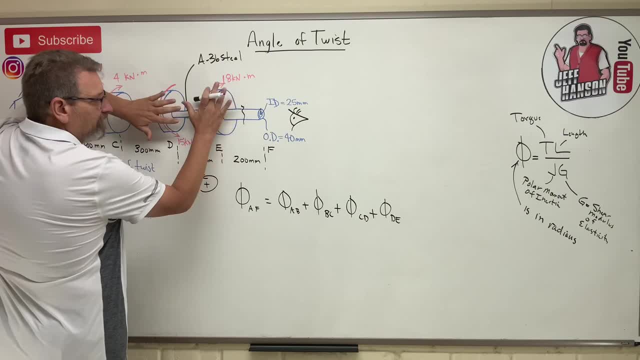 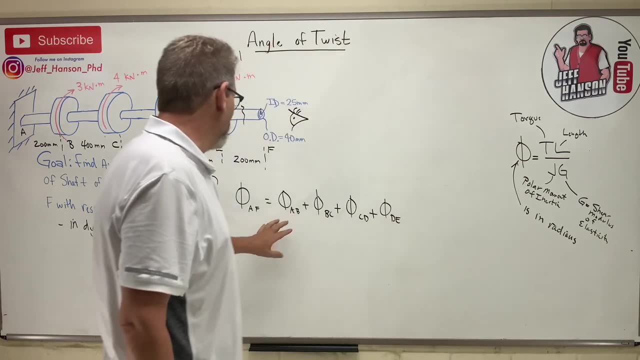 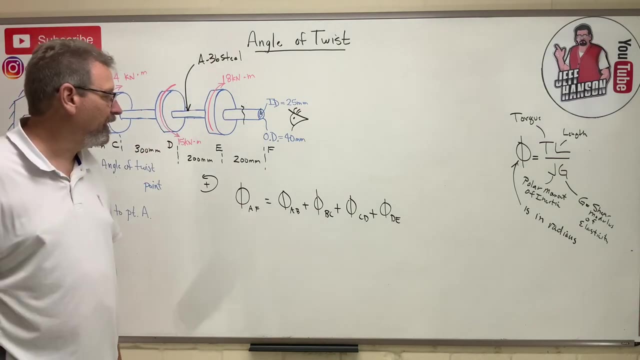 if we cut it in half and we cover all this up, how much torque is in that last section over there, zero. so if t is zero, phi is zero, right? so we've got to add these four things together to get the total with one in from one end with respect to one end of the other. okay, so let's see if we can do. 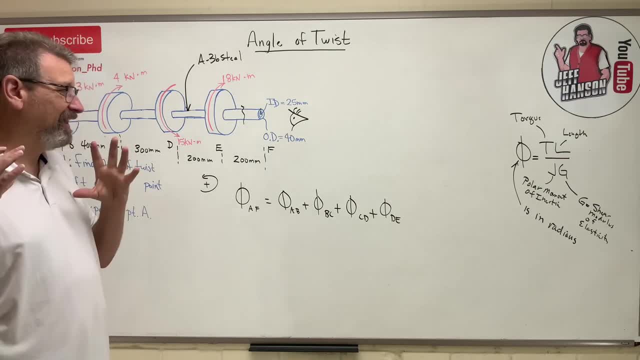 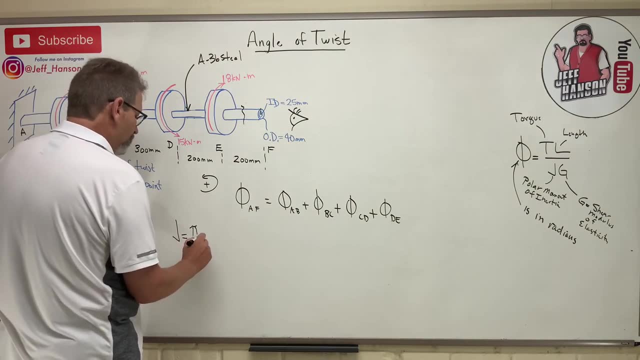 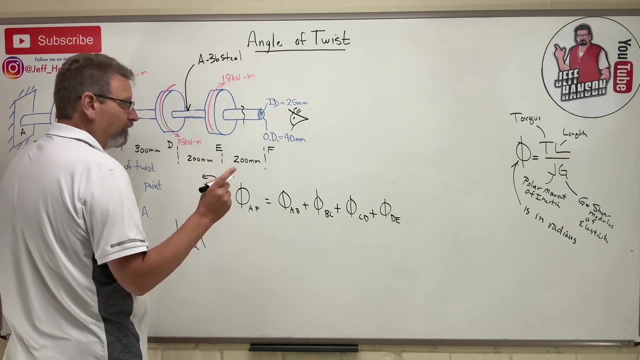 this. let's calculate some things that won't change. okay, j will not change. j is equal to pi over two times. i don't even know. uh, oh yeah, it's r to the fourth and, because i'm at the beginning of the of the outer, minus r to the fourth of the inner, So this is going to be 20 to the fourth minus. 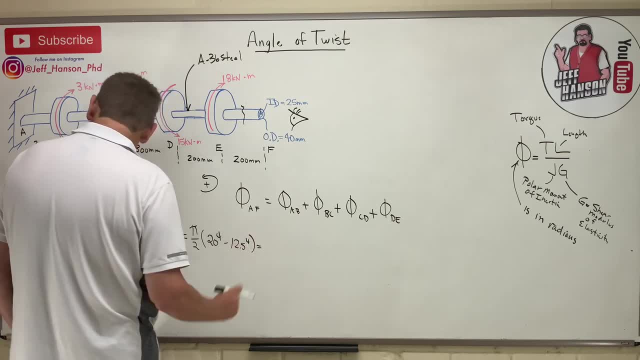 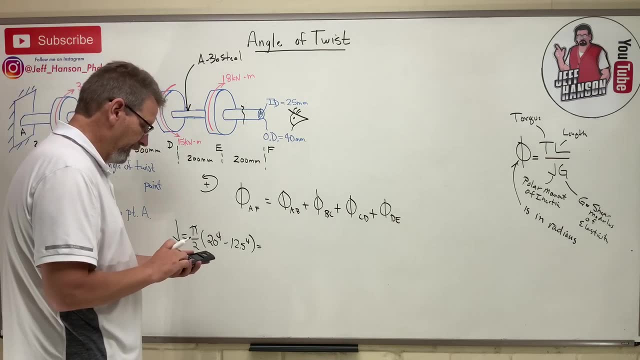 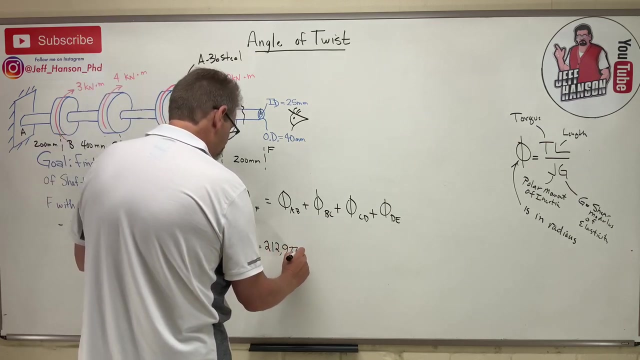 12.5 to the fourth, which equals. where's my calculator? Okay, here we go. Clear: 20 to the fourth minus 12.5 to the fourth equals. and then times: pi divided by two is 212,977.9 millimeters. 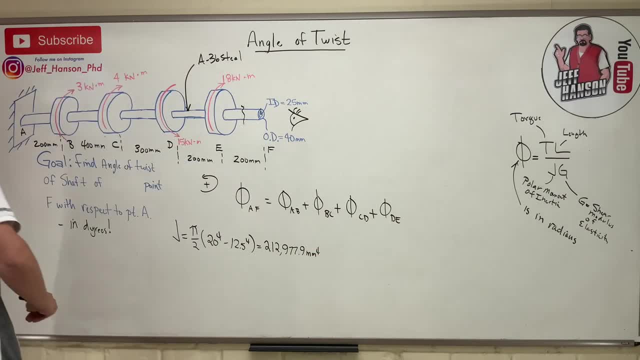 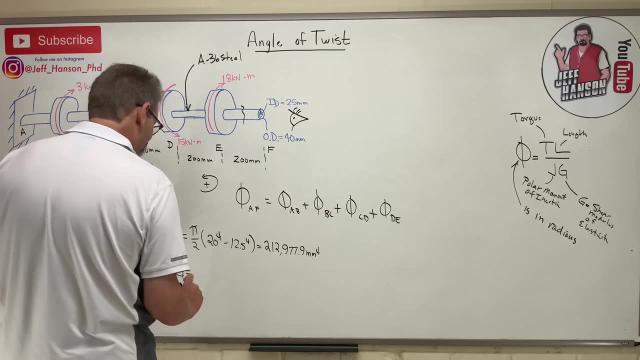 to the fourth. Okay, there's that. Now, what do we have to do? Well, we could get g, couldn't we g? the shear modulus of elasticity. You know what We're going to need? our book right Now. this is: 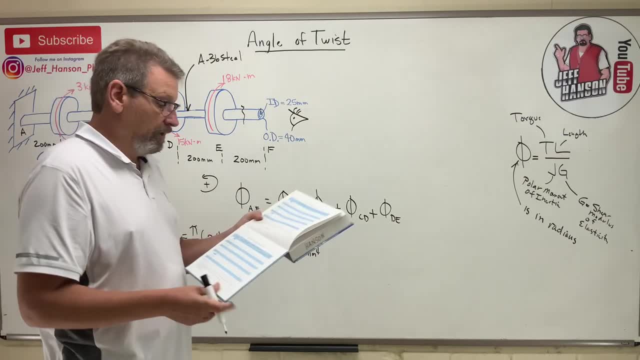 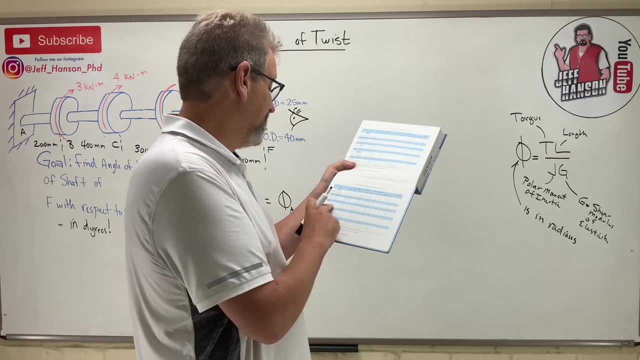 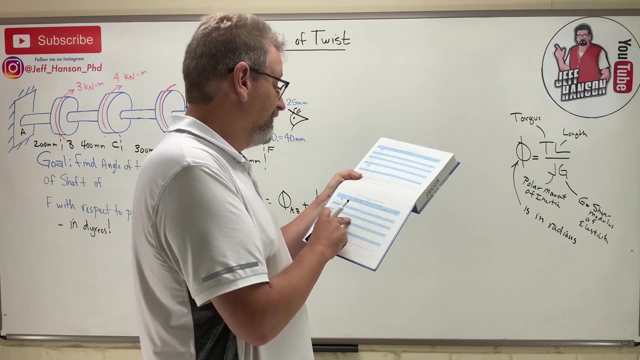 in metric units that we're working with here. So I'm going to go to the SI units table right And I'm going to look up A36 steel- which is where is that Right there, And I'm going to read g just off of my table here And it says g is 75 gigapascals. 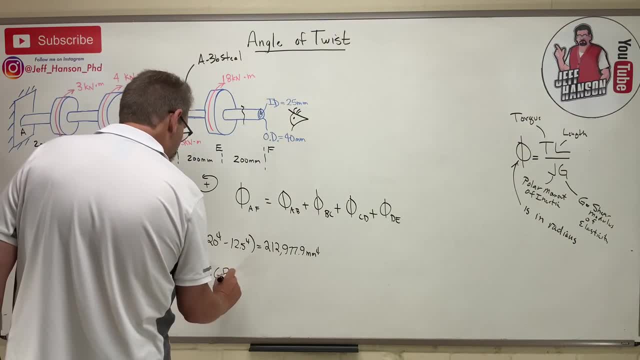 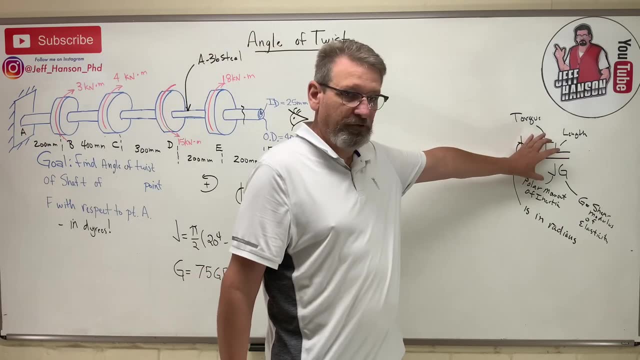 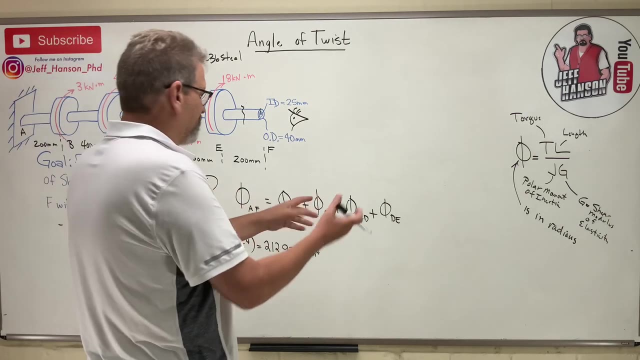 75. 75 gigapascals. Okay, Now I've got to be super careful with my units when I build this equation over here that everything cancels out. okay, The next thing I need is the length of each section- That's easy enough, right, It's just given- is what's the torque in each section? 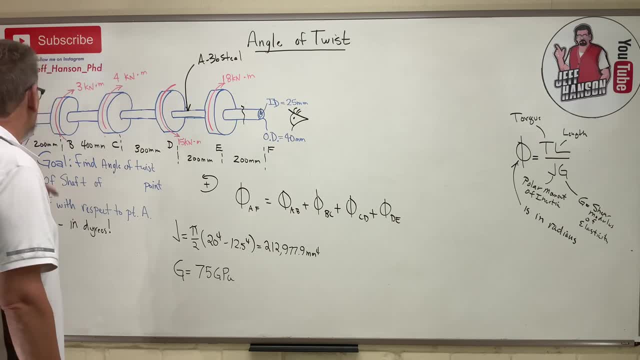 okay, And you can do that by just covering up, right. Okay, so here we go. What's the torque in this section here, in A, B, I don't know. Well, there's a reaction torque at the wall here, right. 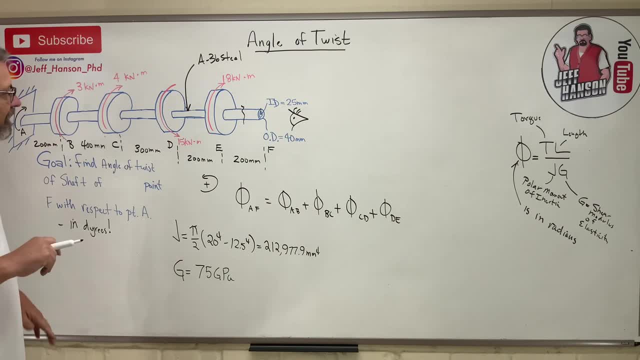 There's some reaction torque at the wall. okay, How big is that and which way is it going? Okay, let's just see what everything's happening over here, okay. So let's do this, Let's cover this up and we'll add all of that up, right? So I got clockwise. I got 3 and 4 and 18.. So that's 7 plus. 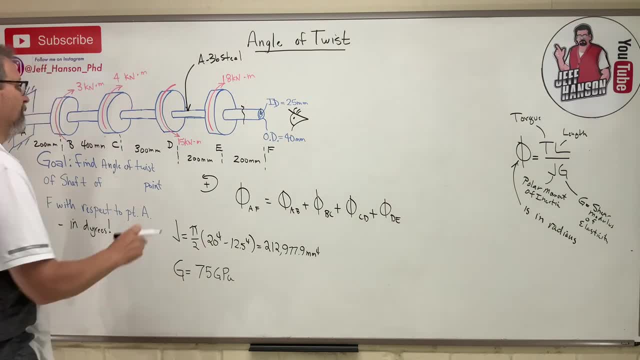 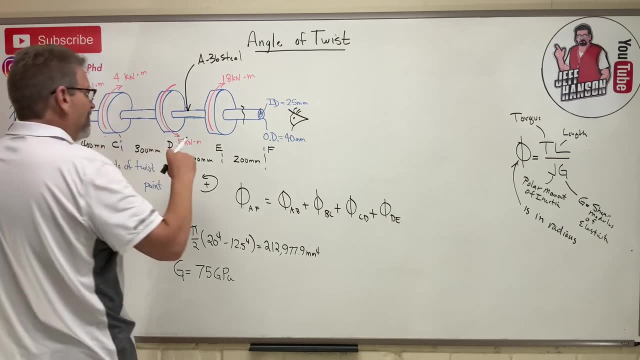 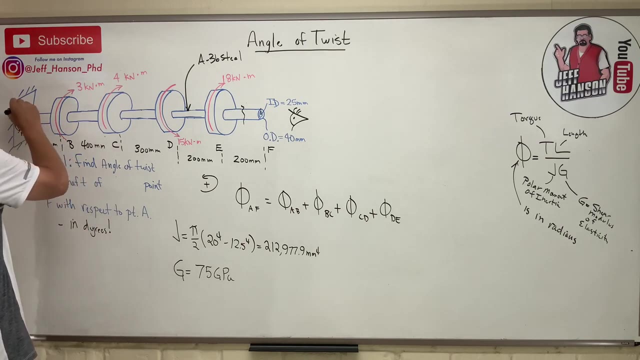 8.. 18 is how much? That's 25 minus 15 nets me 10 clockwise. okay, There's 10 clockwise torque on this section. So this guy has to be 10 anticlockwise, doesn't it? Okay? and that's kilonewton meters, okay. So this section here, 10, and I'm going to say 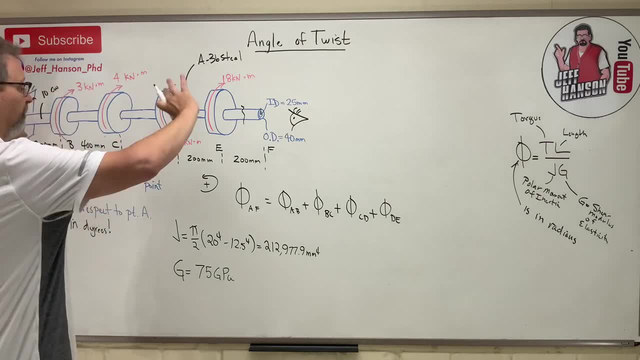 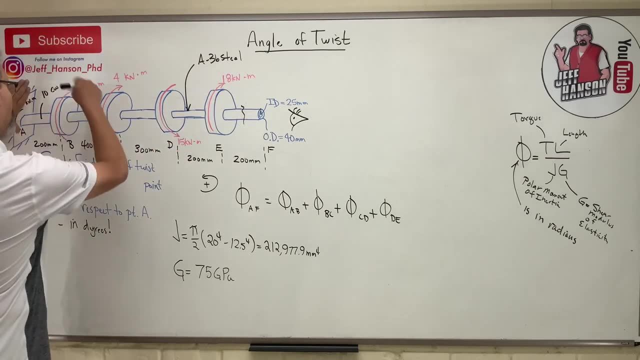 clockwise right, Because all of this, all of this, is a net clockwise right. So it's trying to rotate that one. Leave the wall still right. It's trying to rotate it clockwise, isn't it? Okay, what about? 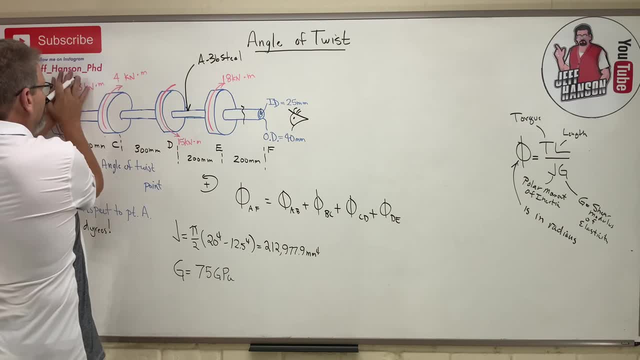 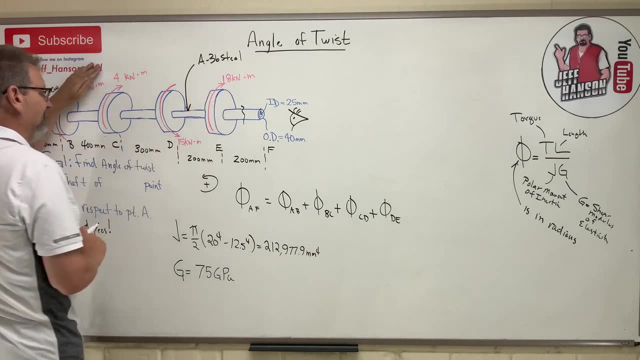 this section of the shaft. okay, Let's cover this up. and what do we got left over here? Well, I got clockwise. I've got 4 plus 18.. That is 22, and then minus 15 leaves me 7.. 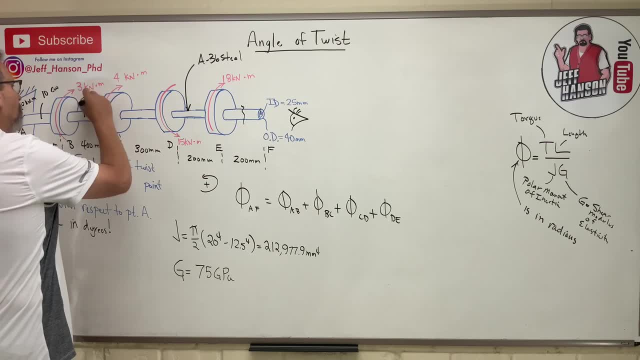 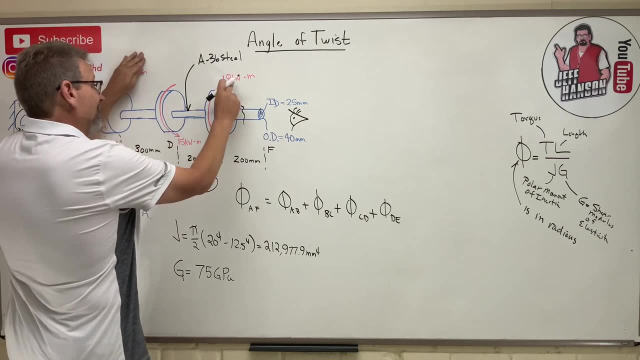 So this section here, 7 clockwise. okay, What about this section? Let's cover this up. What do we got over here? Well, I got 18 clockwise and 15 counterclockwise, which means that this section here has: 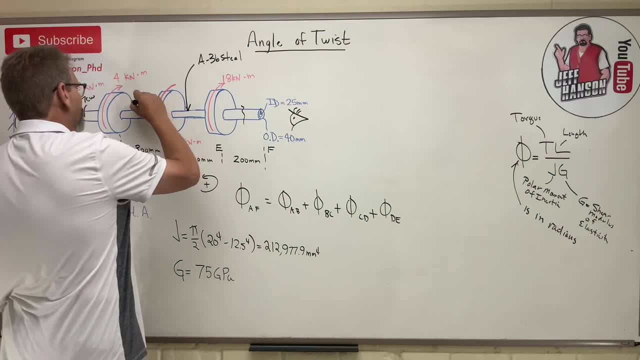 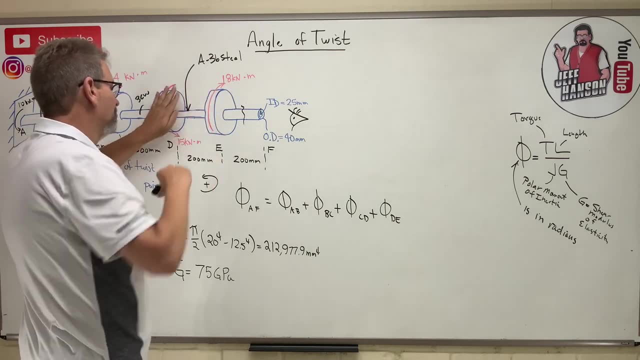 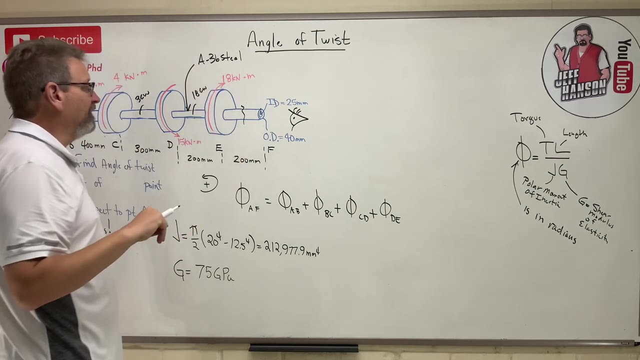 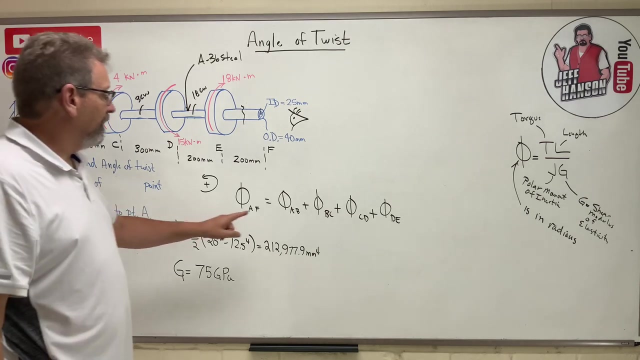 3 clockwise, doesn't it? And then what does this section right here have in it right, Cover all that up. It's got- oh, it's got- 18 clockwise in it, doesn't it? So everything has got clockwise torque in it, right? So I could. I'm going to just 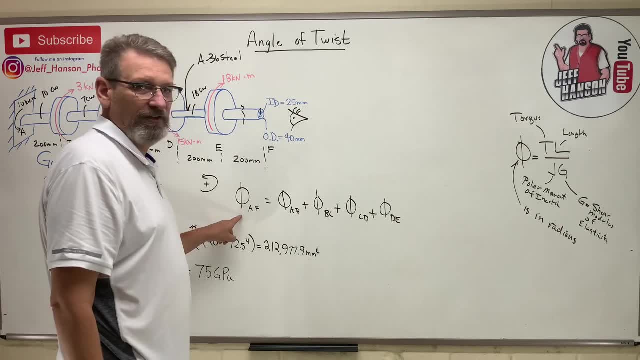 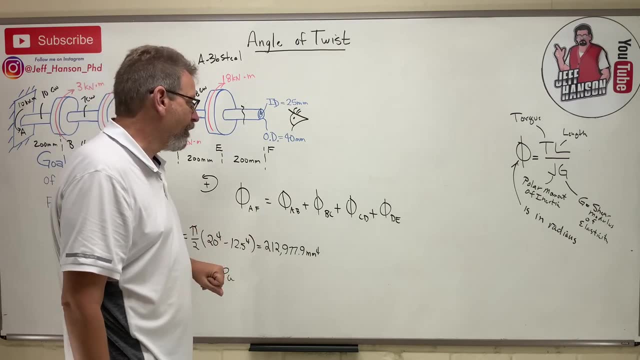 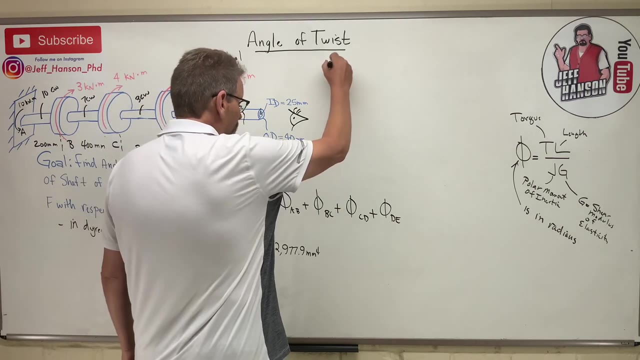 I'm going to leave all these positives right, And I know that AF is going to. the net is going to be clockwise, since that's clockwise, clockwise, clockwise, clockwise. This is going to be clockwise, isn't it Okay? So let's just do these and add them together here, okay? So phi for AB. 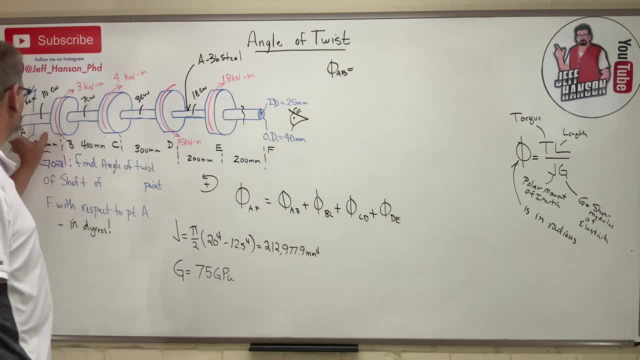 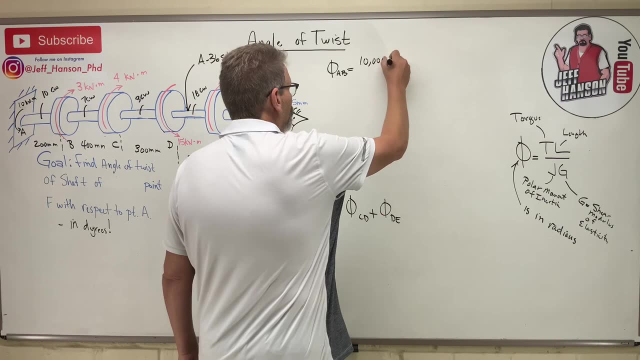 is equal to: okay, AB is way over here. The torque is 10 kilonewton meters, or 10,000 newton meters. okay, I got to get rid of that. got to get rid of that meters, don't I? 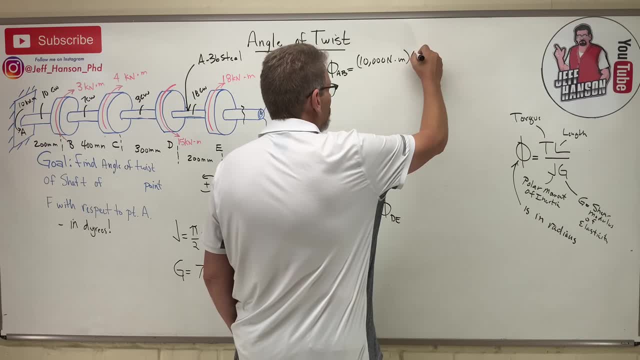 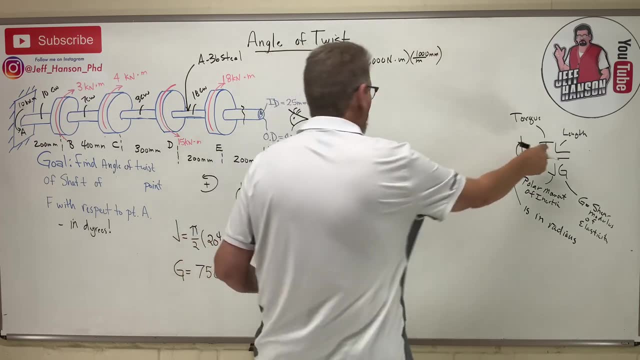 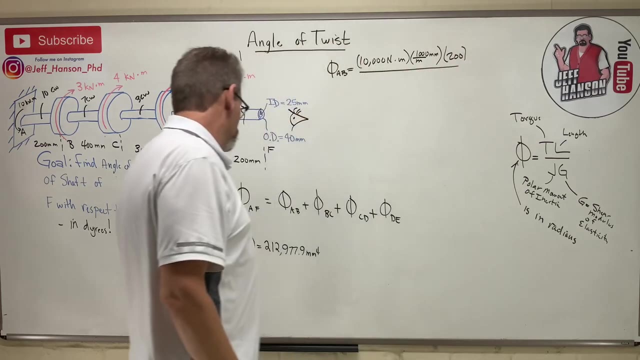 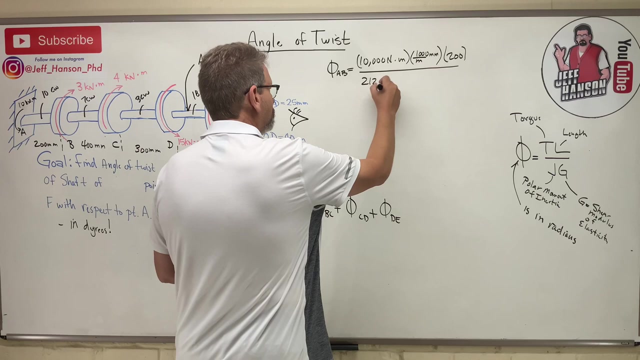 I'm going to turn that into millimeters, right? So that's just going to be times 1,000,, okay, And then times L, that's 200,, okay, Divided by JG, okay. So this guy is going to be in 212,977.9.. That's millimeters. 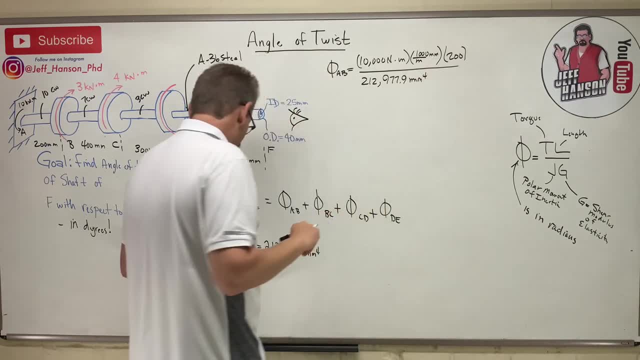 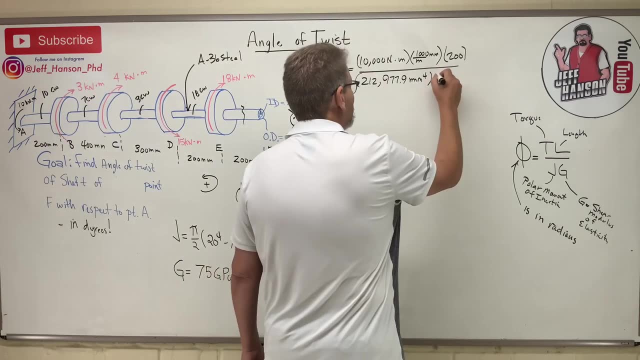 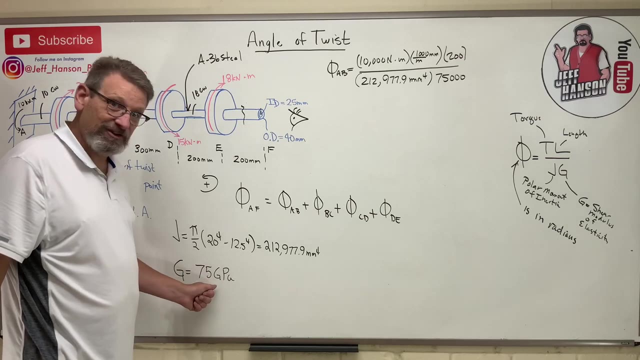 to the fourth And then G. oh, G is in gigapascals. I don't like that. You know what I like. I like this. I like this: 75, 1,, 2,, 3, right, If I take three, put three more zeros on there, that goes from a giga to a mega, And hey. 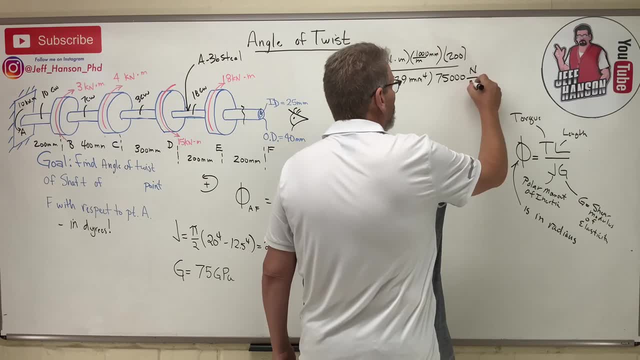 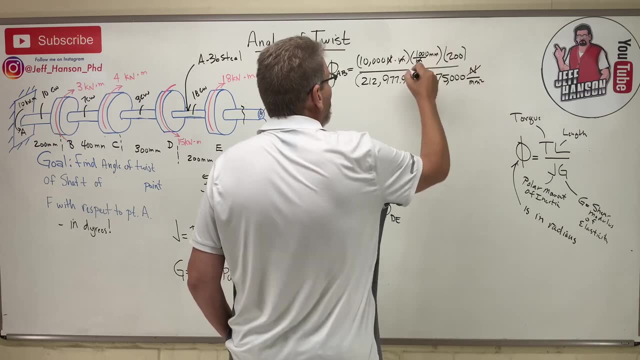 I know what a mega is. A mega is a newton divided by millimeters, squared right. And now let's see if everything cancels out. I got a newton and a newton, a meter and a meter. This is in millimeters. 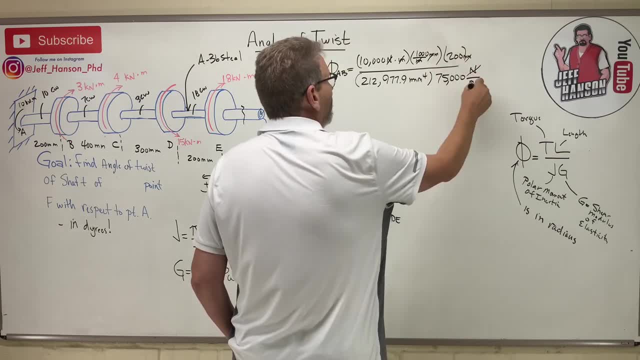 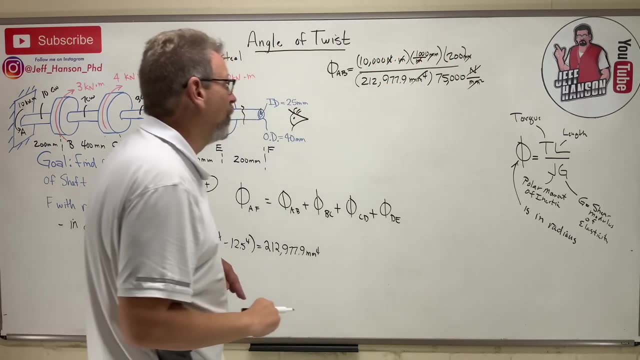 right, I got two millimeters And then I got two more that go to the top, So that makes four millimeters, And then there's four there, bam, bam. all of it cancels out, right. So I got no. 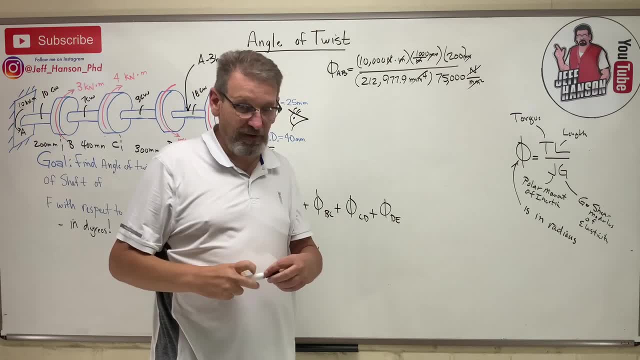 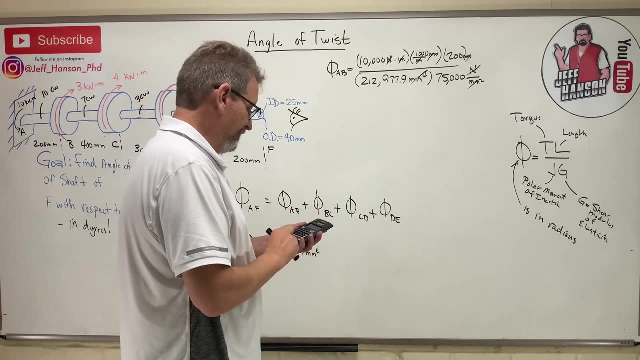 left. I feel good about this. I know that my calculation is going to be right. Let's see what it is. Okay, here we go: 10,000.. Now remember, this is going to be in radians Times, 1,000. 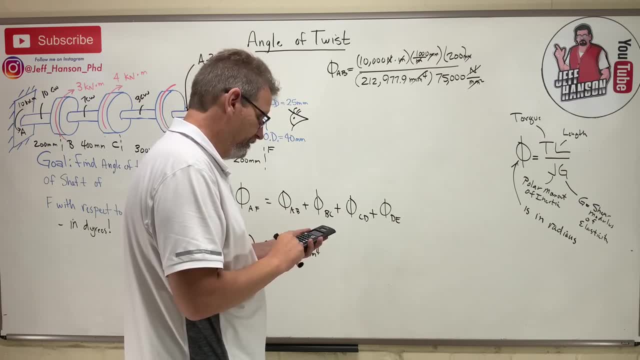 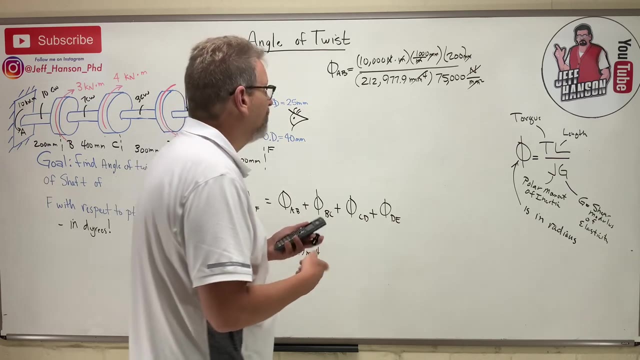 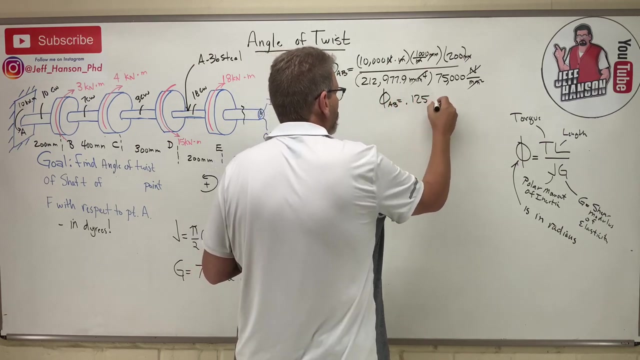 times 200, divided by 75,000, and then divided by 212,000.. 977.9 equals 0.125.. So phi AB equals 0.125.. Totally rad man. Okay, that's the first one. 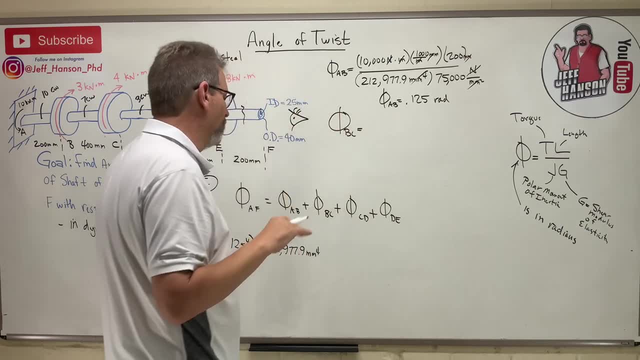 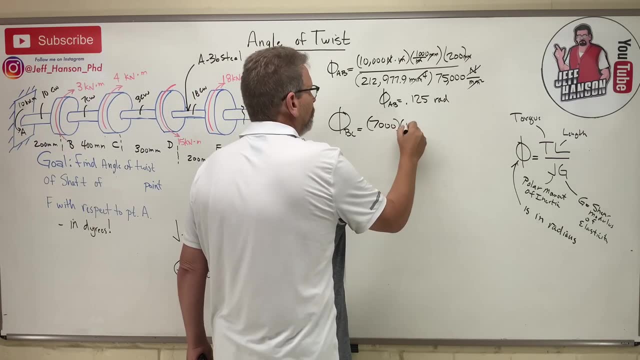 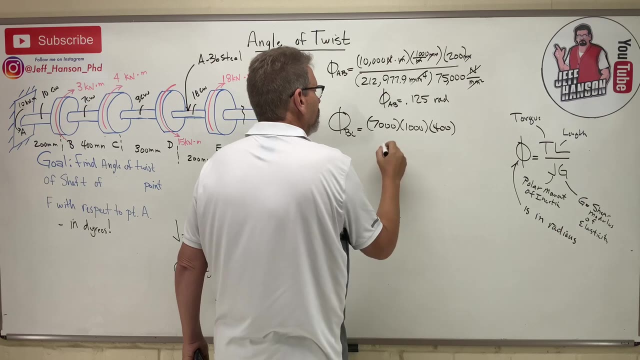 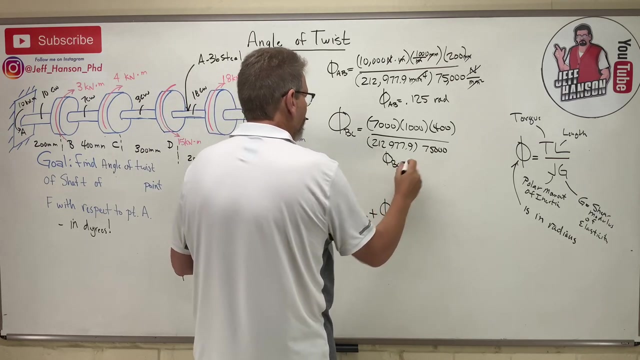 phi BC. Okay, we can go faster. Now we know what. everything is right. The torque is seven, So that's 7,000 times 1,000 times the length, which is 400, divided by 212, 977.9 times 75,000.. Okay, so phi BC, phi BC is 7,000. 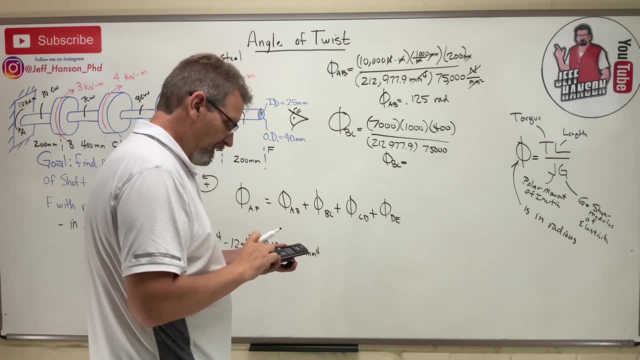 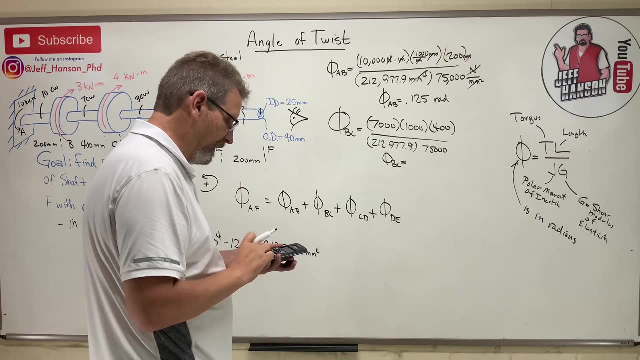 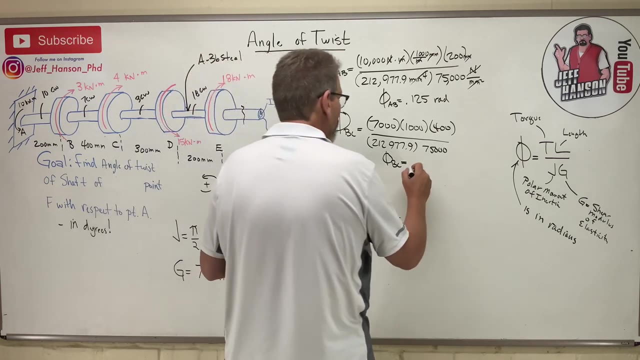 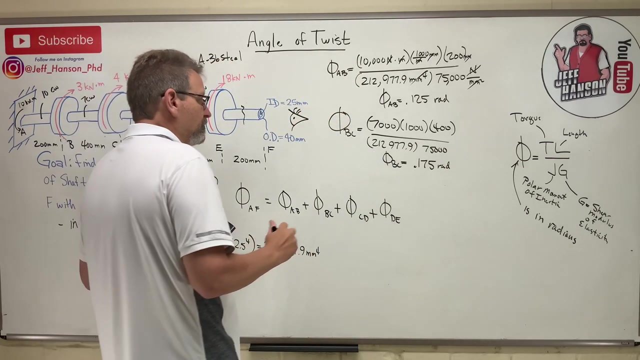 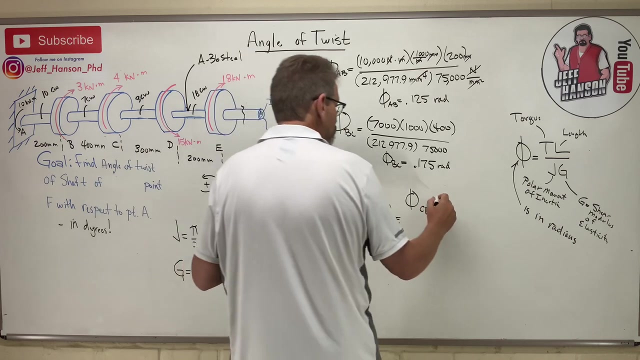 times 1,000 times 400, equals divided by 212,000.. 977.9 divided by 75,000, 0.175.. Okay, and then finally- well, not finally. we got two more to go. we've got to do phi. CD, which is going to be the torque, is three, So that's 3,000 times 1,000 times. 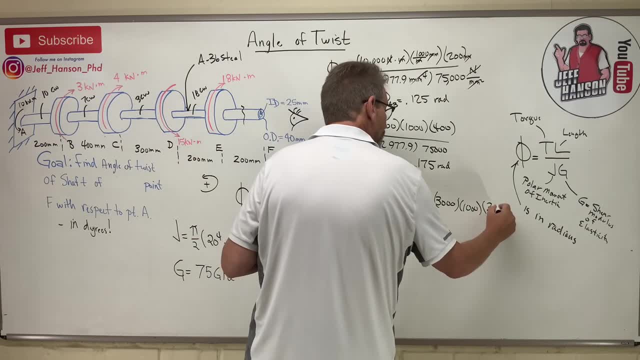 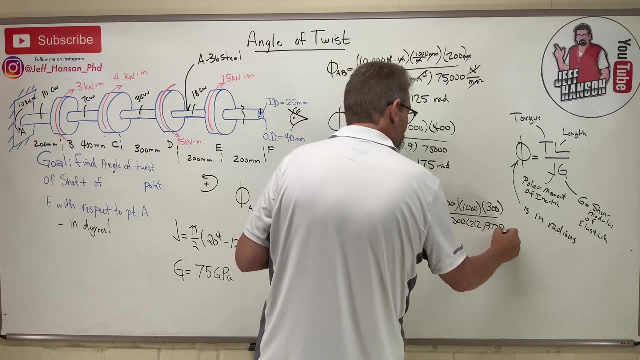 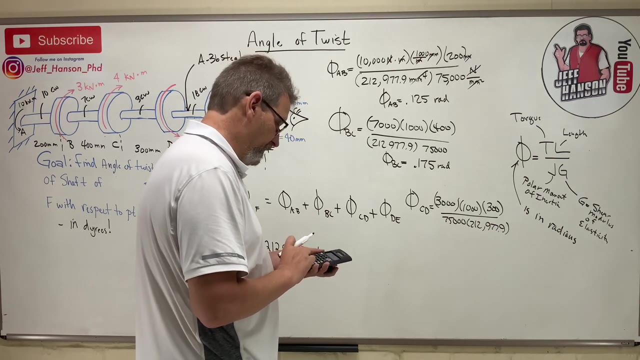 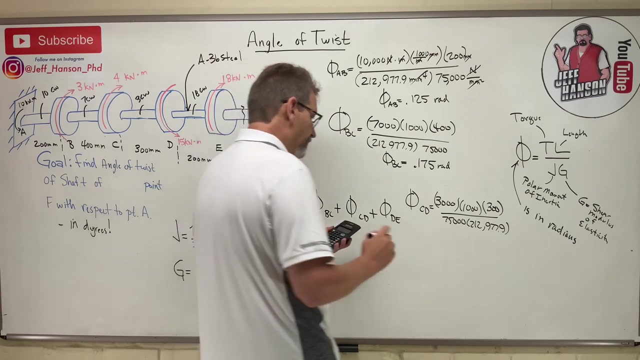 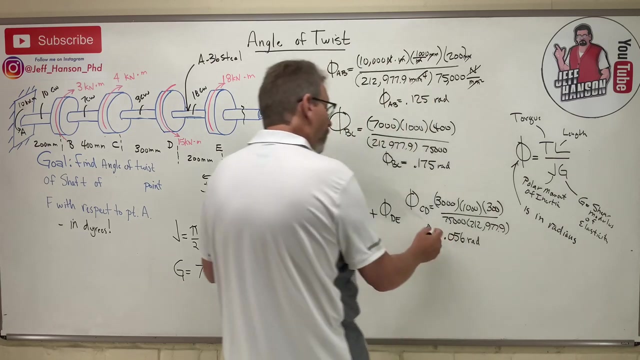 the length CD 300, divided by 75,000 times 212,977.9.. So that one is times 1,000 times 300, equals divided by 75,000, divided by 212,977.9.. 0.056.. Okay, well, why is that one so much smaller than those? Well, because the torque is so much. 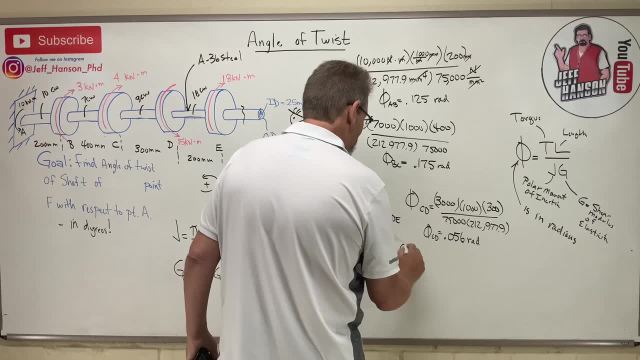 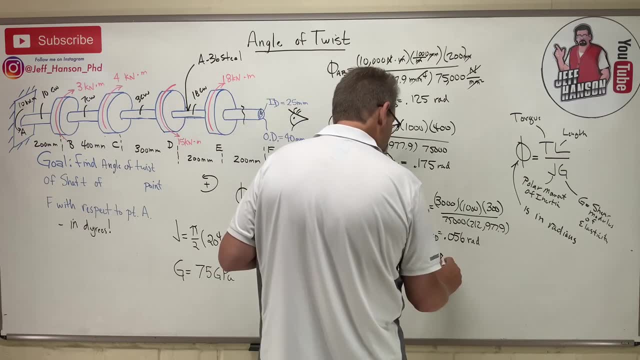 smaller right? Yep, Okay, and finally, phi DE is equal to what do we got Over here? we got 18,000 times 1,000 times 1,000 times 212,977.9.. So that's 3,000 times 1,000 times 212,977.9.. 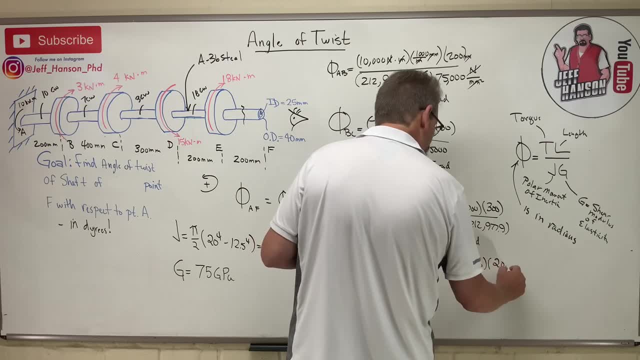 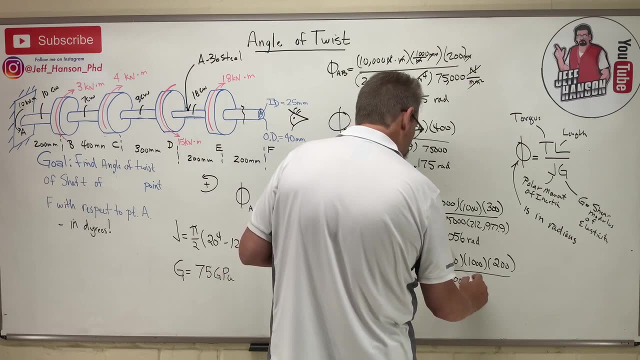 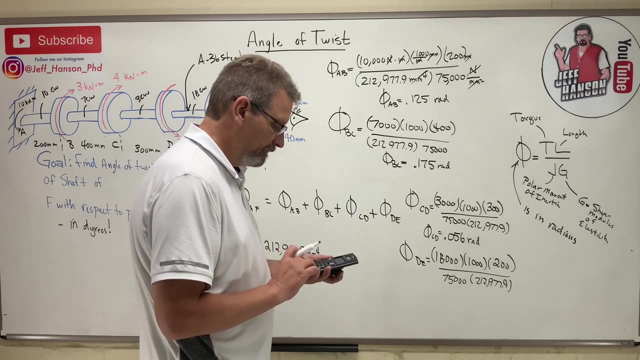 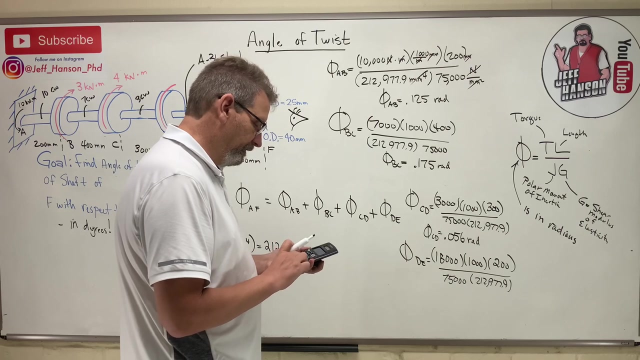 What's that guy? 200 divided by 75,000 times 212,977.9.. All right, here we go one more time. 18,000 times 1,000 times 200, equals divided by 75,000. divided by: 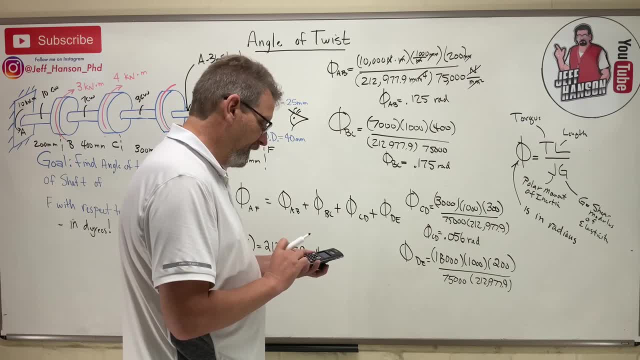 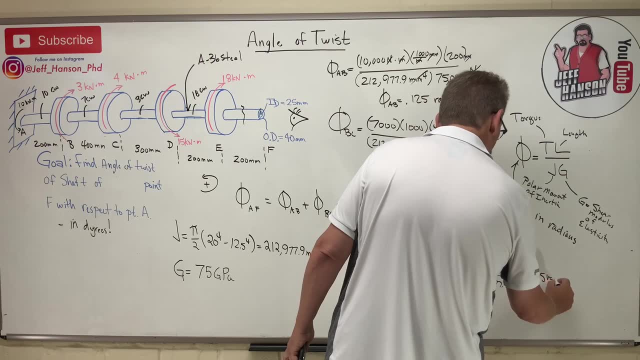 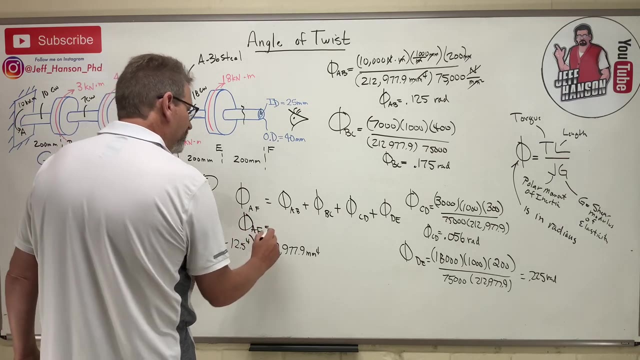 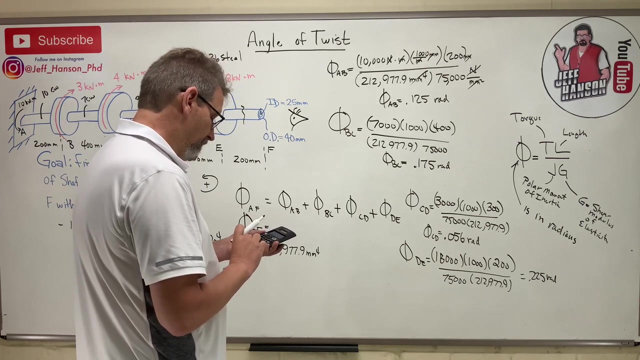 75,000 times 212,977.9, 0.225.. Okay, so the total deflection phi A to F right is going to be that one plus 0.175 plus 0.125 plus 0.056.. Don't forget about that: 0.056 is going to be. 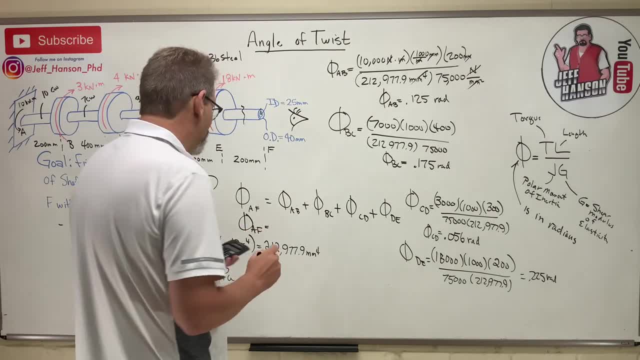 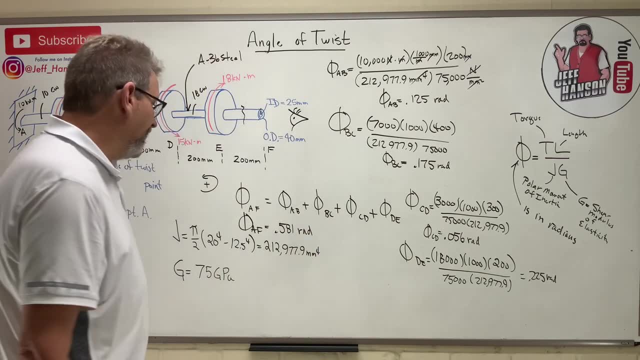 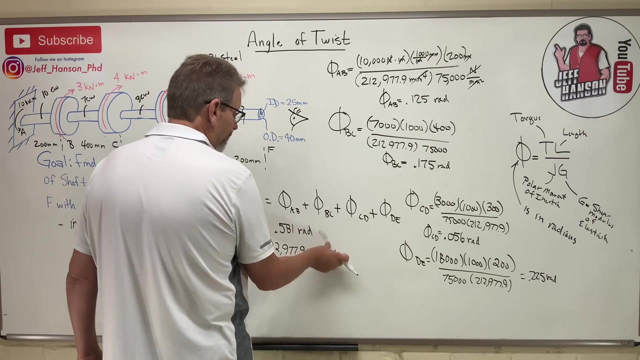 that guy equals 0.581 radians, right? And what if we wanted that in degrees? Okay, now that's going to. oh, I should, I should put. you need to put this on there to be clear, right, That that is. 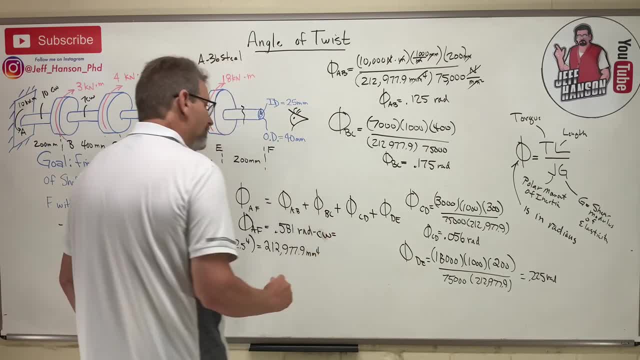 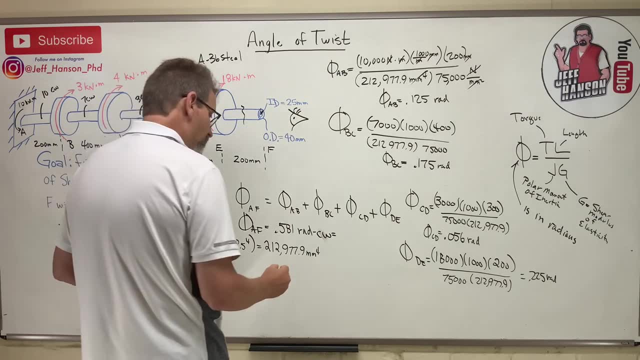 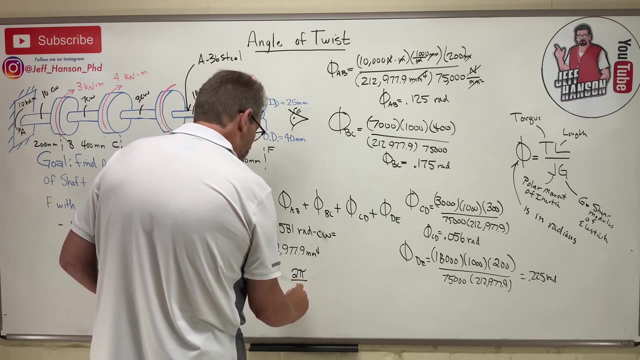 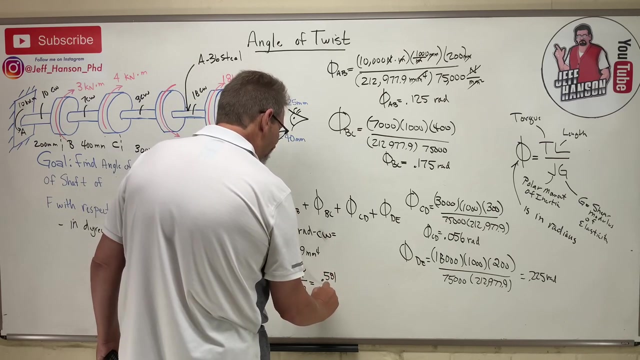 a clockwise rotation, right? So that thing is rotating. Now my little indicator is over there somewhere, right? So how do I convert that to degrees? Here we go: 2 pi is to 180, as that's radians. right, As 0.581 radians is to x degrees, okay, So. 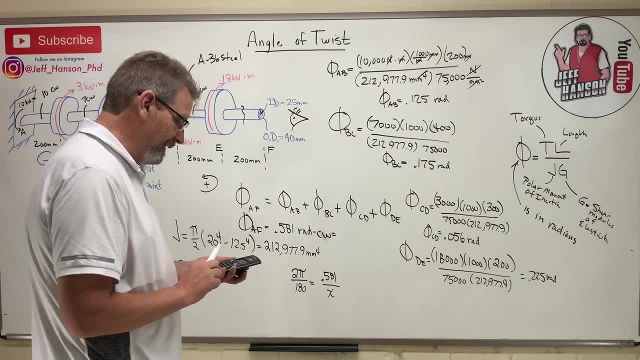 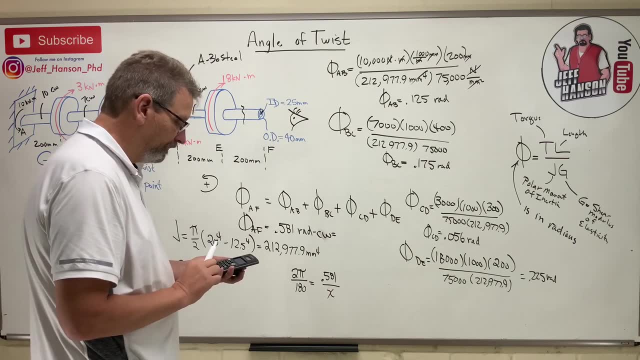 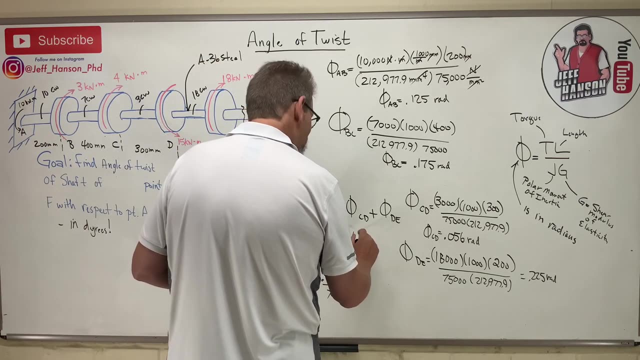 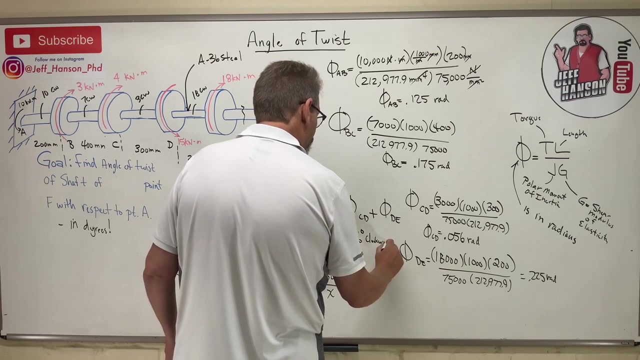 0.581 times 180. equals divided by 2. equals divided by pi pi. where's pi? Pi equals degrees, Six degrees Clockwise. Okay, There you go. So that thing is going to rotate quite a bit.